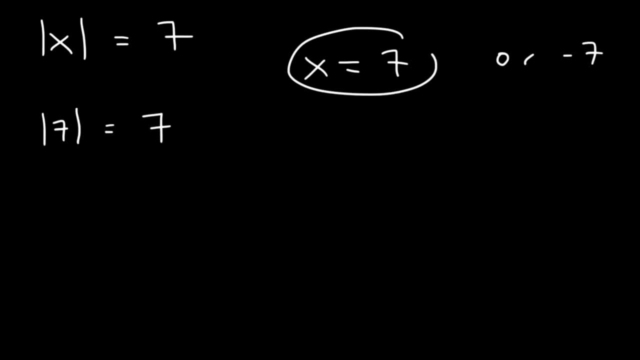 The absolute value of seven is seven, so this works. The absolute value of negative seven is also seven, so X can be seven or negative seven. Both will make the equation true. So now, how can we use this to solve a typical problem that involves an absolute value symbol? 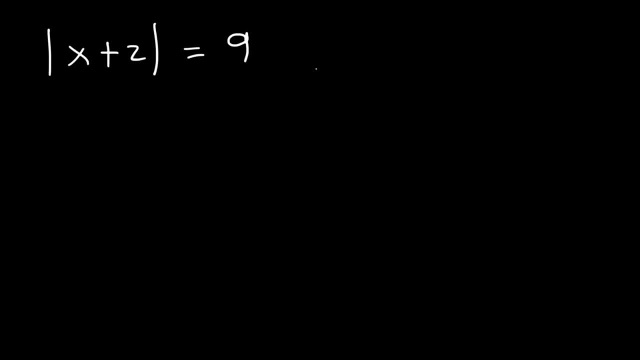 So let's say, if we have the function, the absolute value of X plus two is equal to nine. How can we solve this equation? Well, the first thing you should do is write two equations: the original one and another one where the inside function is equal to negative nine. 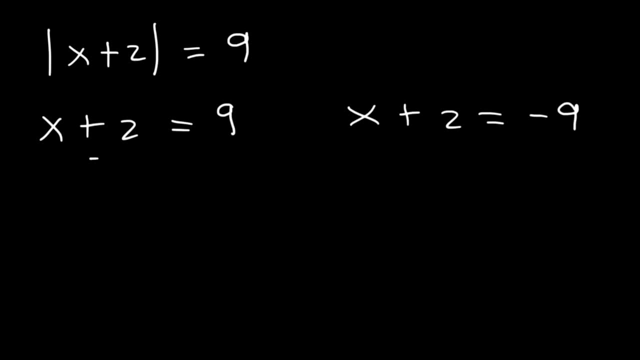 instead of positive nine And solve for both. So in the first one we can see that X can be equal to seven And for the second one, X is equal to negative eleven. So these are the solutions. Find the value of X given this equation. 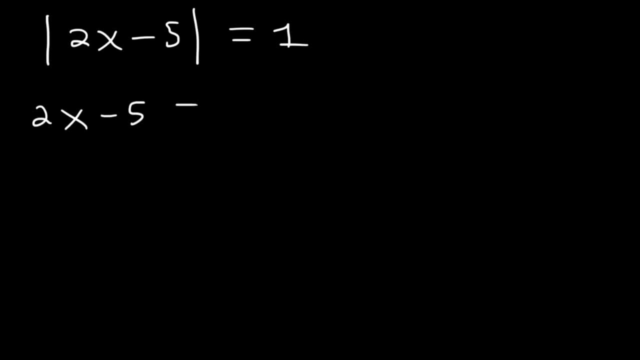 So, just like the last example, let's set two X minus five equal to one And negative one. So first let's add five, One plus five is six, And then let's divide both sides by two, So X is equal to three. 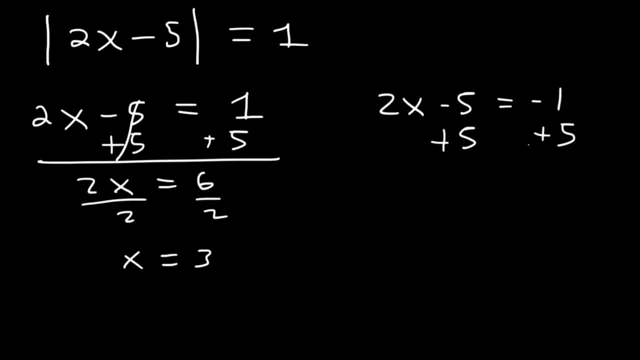 And in the other example let's add five to both sides. Negative. one plus five is four And then divide by two. X is two. So if you check the work you can see that it's going to work out. So if we plug in two, 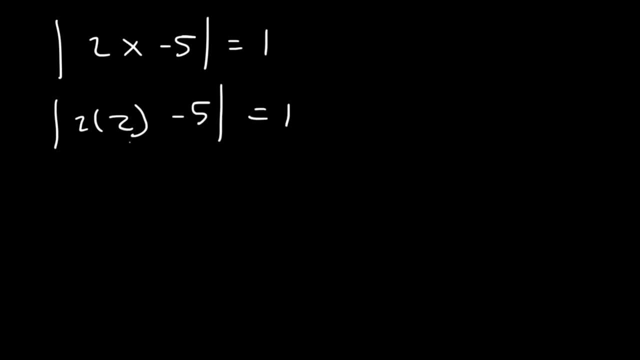 Two times two is four. Four minus five is negative one. The absolute value of negative one is one. So the equation is true. Now if we plug in three, it should also work. Two times three is equal to six. Six minus five is one. 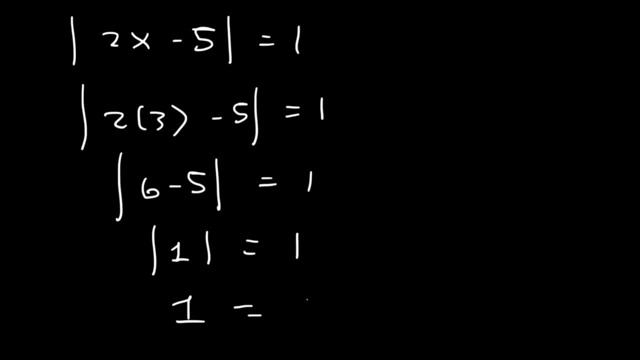 The absolute value of one is one, So that works. Now what about this one? The absolute value of five X minus one is equal to negative two. What's the solution? The absolute value function can never equal a negative number, So there's no solution for this particular example. 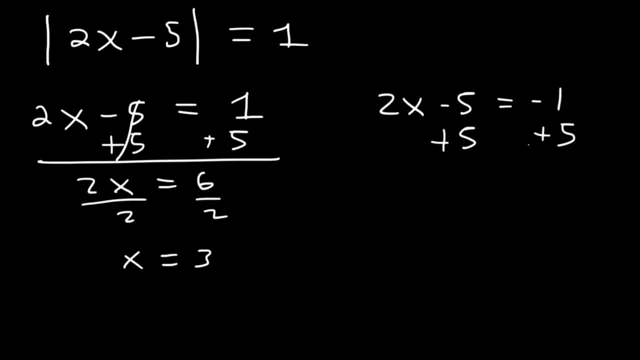 And in the other example let's add five to both sides. Negative. one plus five is four And then divide by two. X is two. So if you check the work you can see that it's going to work out. So if we plug in two, 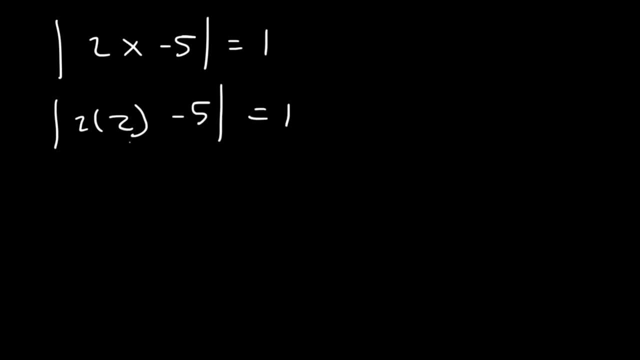 Two times two is four. Four minus five is negative one. The absolute value of negative one is one. So the equation is true. Now if we plug in three, it should also work. Two times three is equal to six. Six minus five is one. 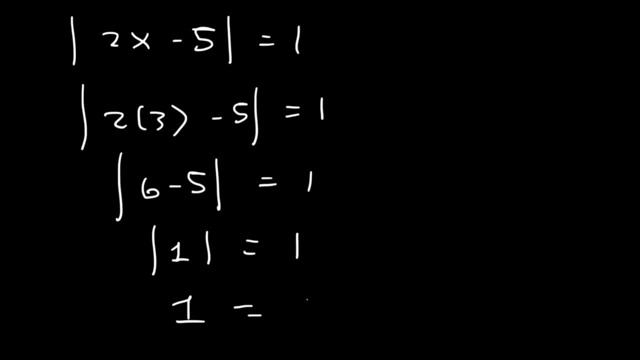 The absolute value of one is one, So that works. Now what about this one? The absolute value of five X minus one is equal to negative two. What's the solution? The absolute value function can never equal a negative number, So there's no solution for this particular example. 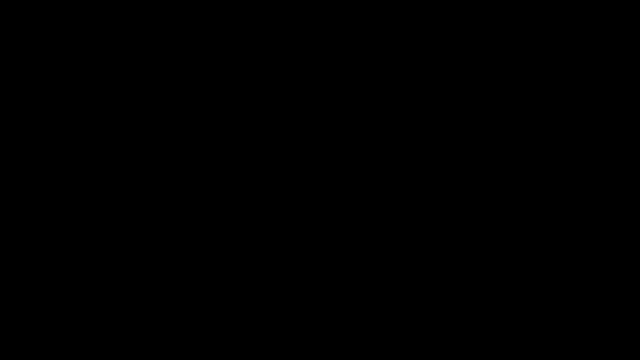 It can only equal zero or a positive number. Now, let's try this again. Now let's try one more example for this particular lesson. Find the value of X. Now, what you don't want to do is write this. equation on the left is equal to seven or negative seven. 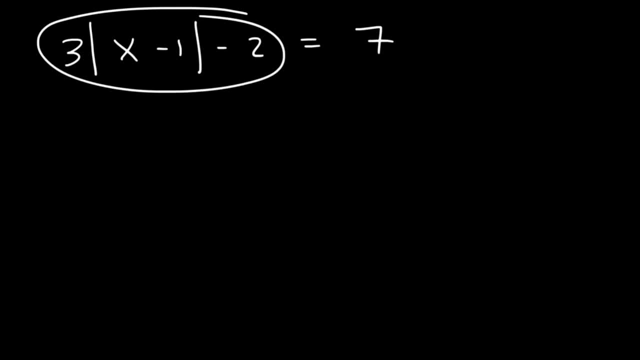 First you want to modify the equation. You want to get the absolute value function by itself. So let's add two first, So we're going to get nine on the right side. Next, let's divide by three. Now you want the absolute value symbol by itself on one side. 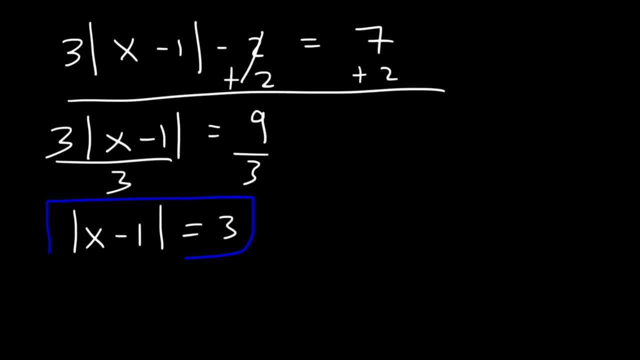 Once you have it. at this point now, you want to write two equations, So the first one is going to be: X minus one is equal to three, And the second, X minus one, is equal to negative three. So if we add one, X is equal to four. 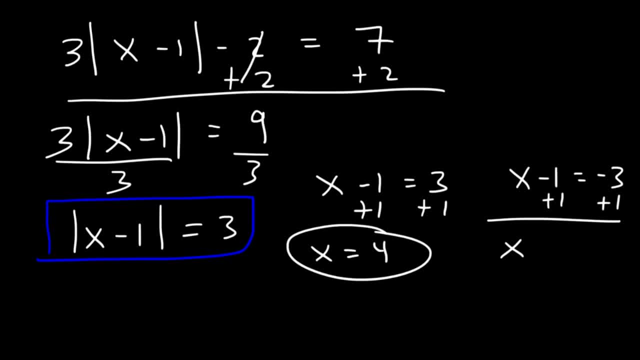 And if we add one to the other, one negative three plus one is negative two. So this is the solution.